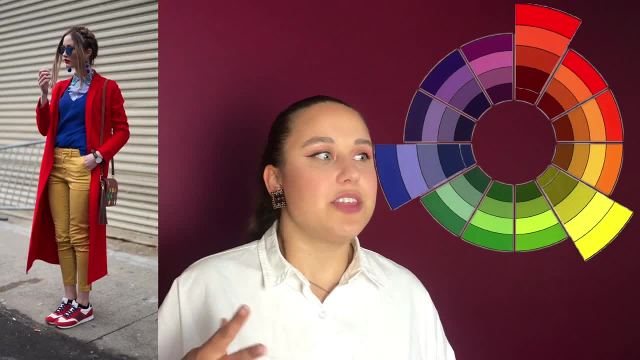 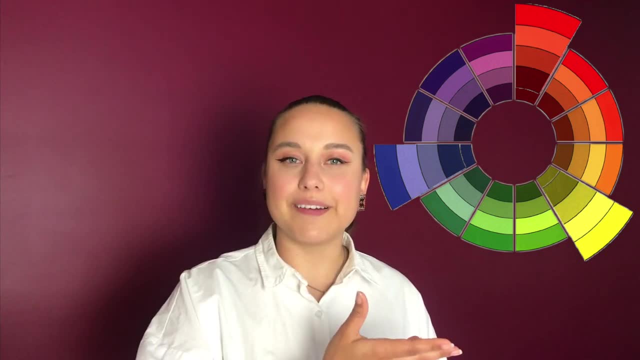 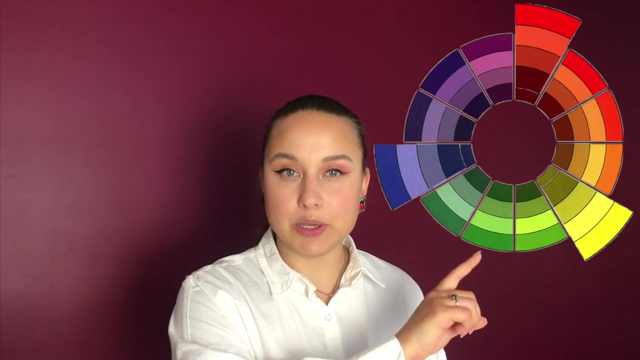 colors are like, they cannot be mixed. They exist. They're the primary colors, So the primary colors. they cannot be made out of different colors. So here they are Now. if we mix yellow and blue, then we'll get green. If we'll mix blue and red, we'll get purple. And if we mix yellow and red, 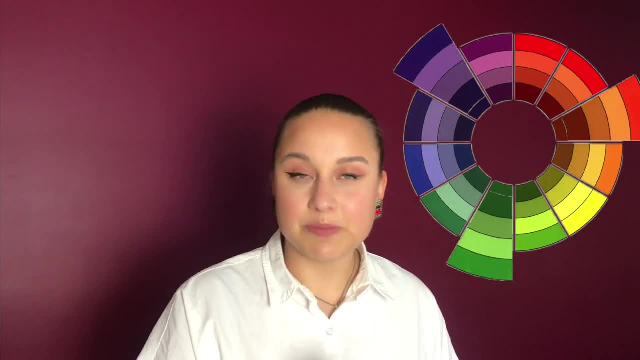 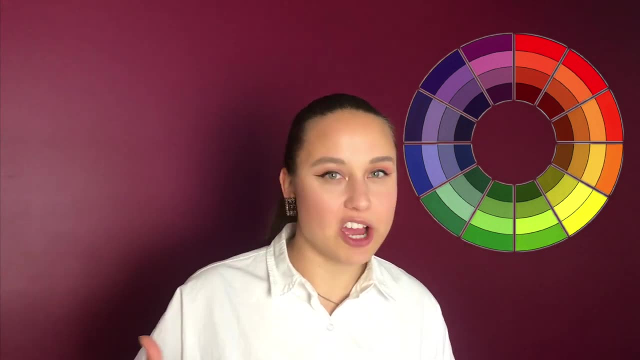 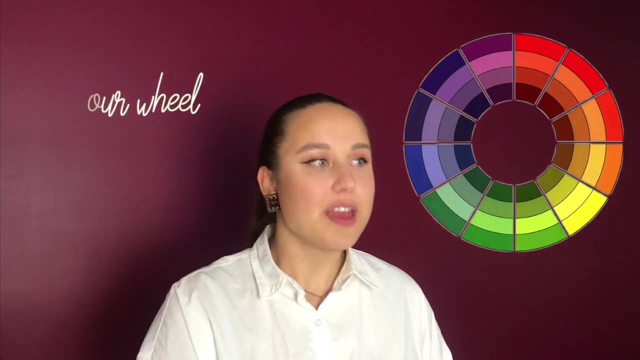 we'll get orange. These are the secondary colors. Tertiary colors are the ones that are kind of fit in between those, everything else. Now let's talk about the warmer and the cooler side of the circle, Color circle. Yes, So the warmer colors will be the yellows, the oranges, the reds. 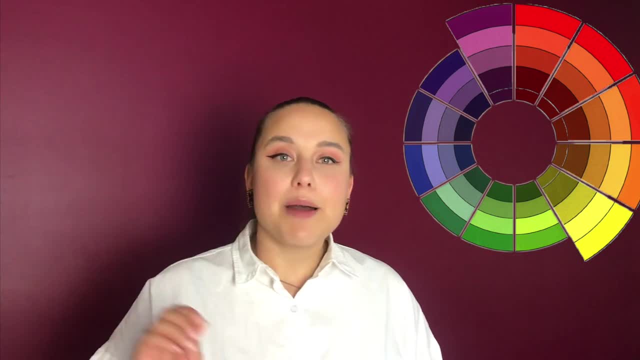 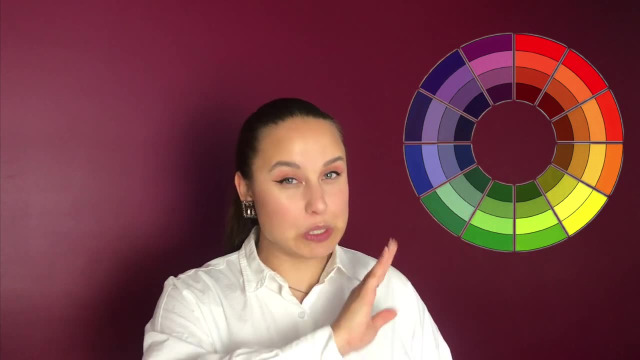 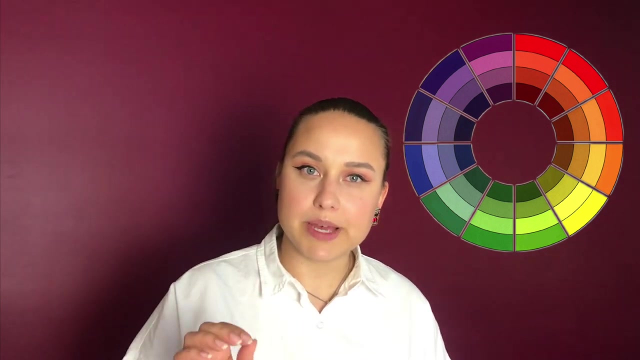 maybe some of the green And the cooler tones would be the purples, the blues and kind of like the greenish blues. So depending on your color tone then you can figure out which colors work best for your skin tone. All right, Now, every color. 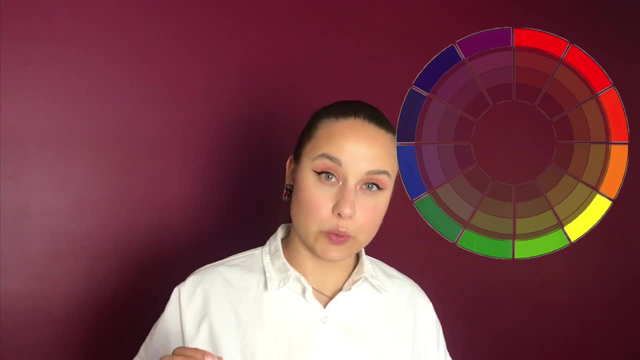 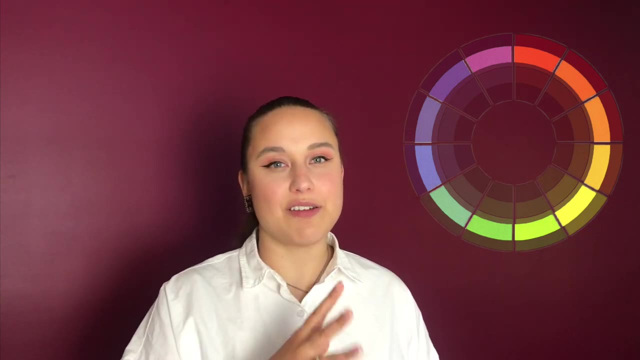 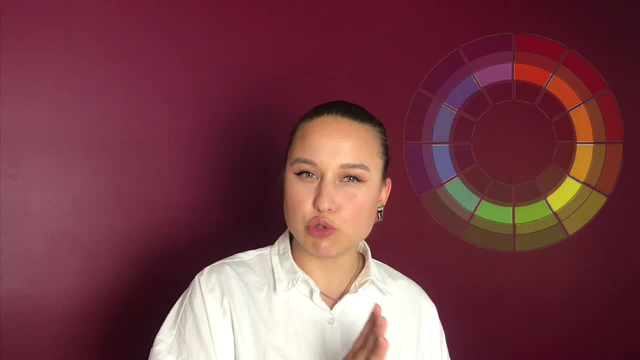 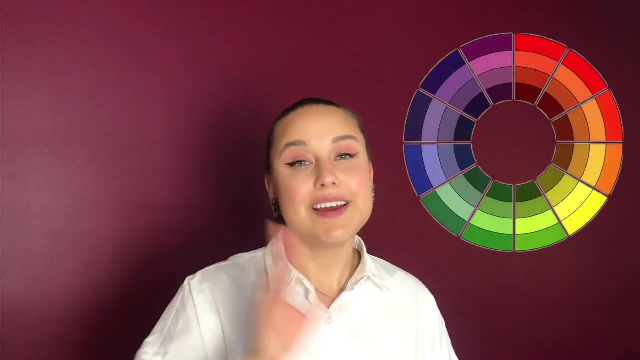 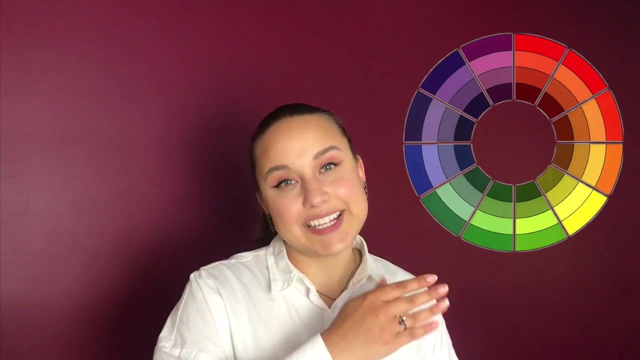 kind of dilute it with a gray, making it more neutral. it would be a tone. Okay, Now that we've got all of that out of the way, let's talk about what colors like go together with what. So in opposite sides of the circle we see complementary colors. Why are they called? 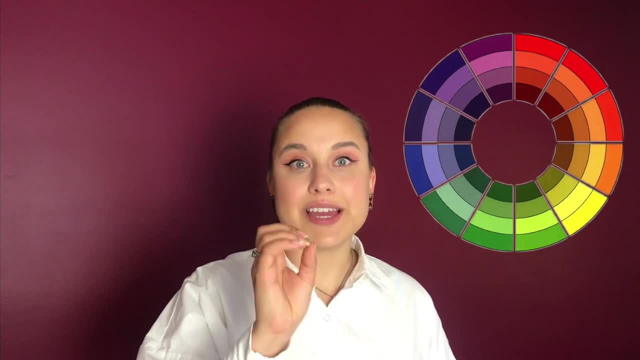 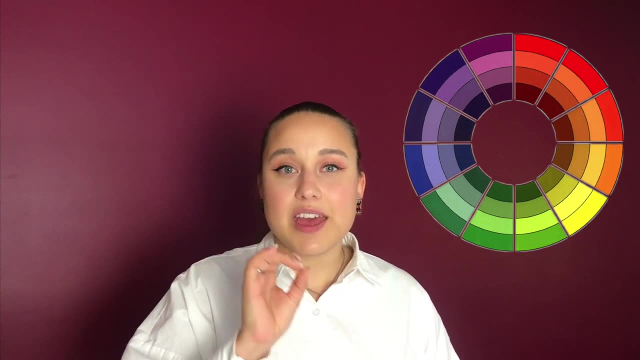 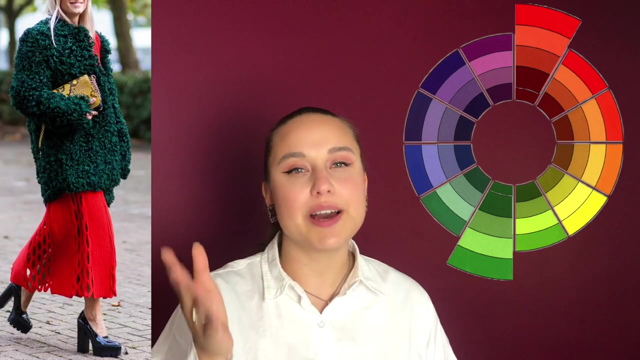 complementary colors is because when they're put together the eye they kind of highlight each other, So they're really really bright pairing. So, for instance, the green and red are actually complementary colors. So that's why we have the Christmas: it's green and red and super bright. 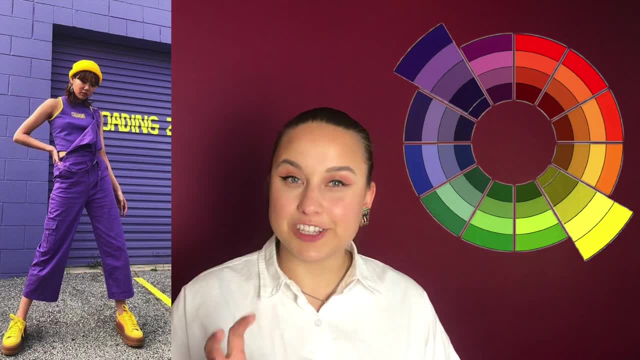 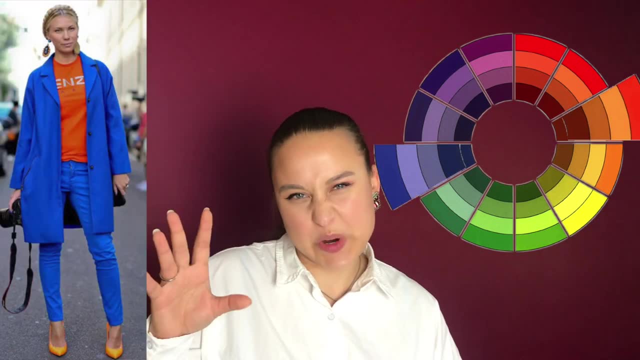 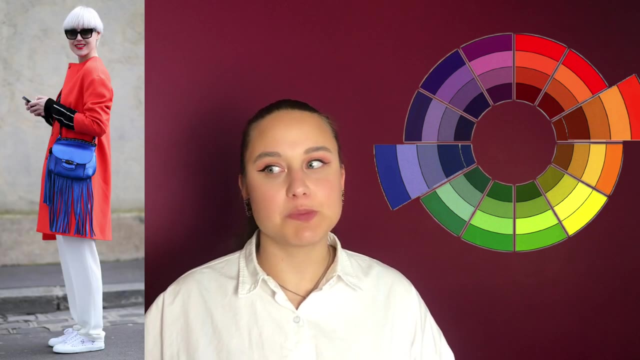 Yeah Yeah, Yellow and purple are really kind of a toxic mix as well, as well as the blue and yellowish orangish color. So now that we figure out like what, like either we want to follow those just because they're super bright or we want to stay away from them because it is your choice, right, If you don't? 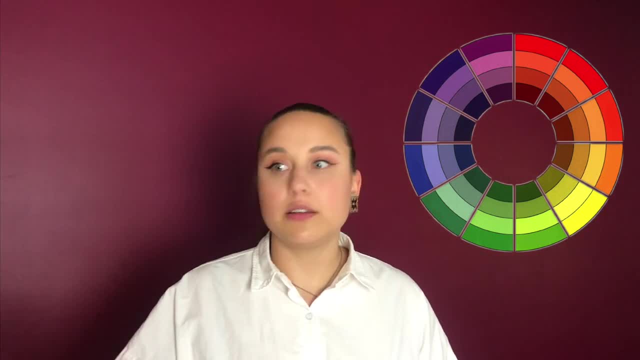 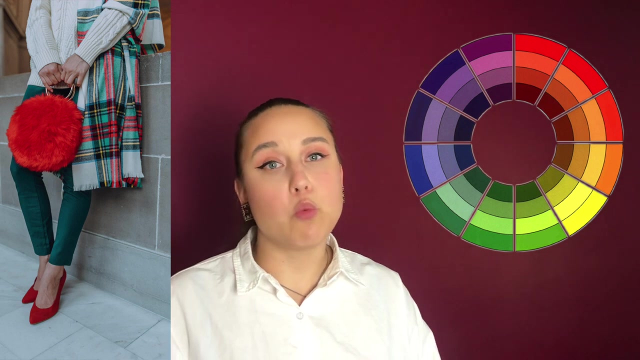 want to be super bright and out there, then yeah, don't do it. And of course, you don't have to wear like huge, like amounts of those colors together. If they're complimentary, you can wear like, for instance, a red pant. you can wear a white shirt with a green necklace. The fact that they're not together, 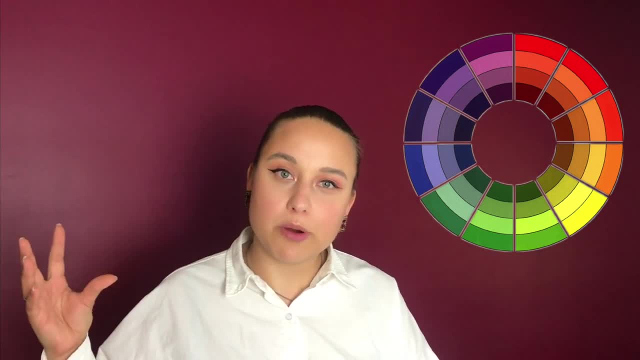 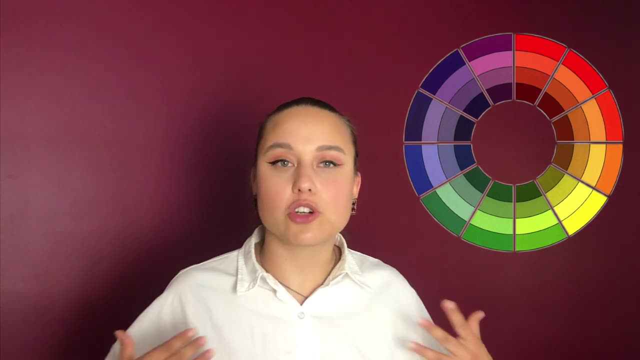 is going to kind of pull them apart and they're not going to stand out as much. Also, you can, maybe the shirt would be with little polka dots of green. So that's not going to be. I don't know. I don't know. 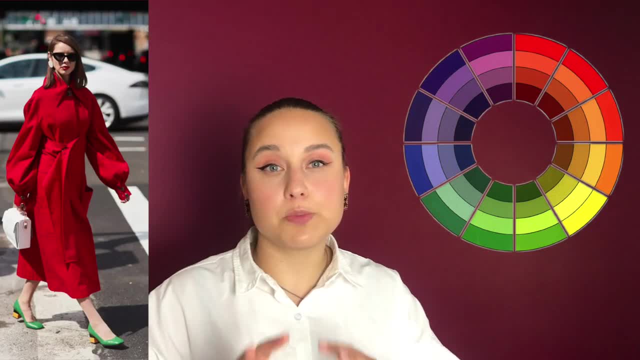 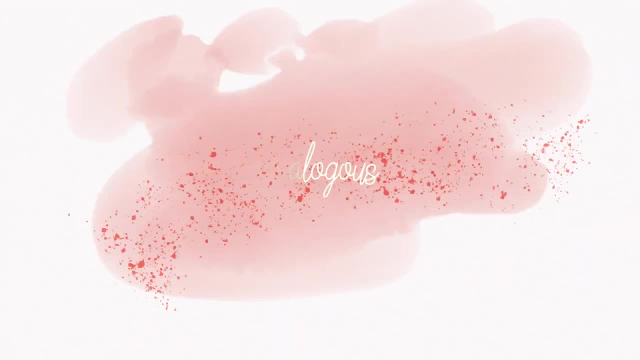 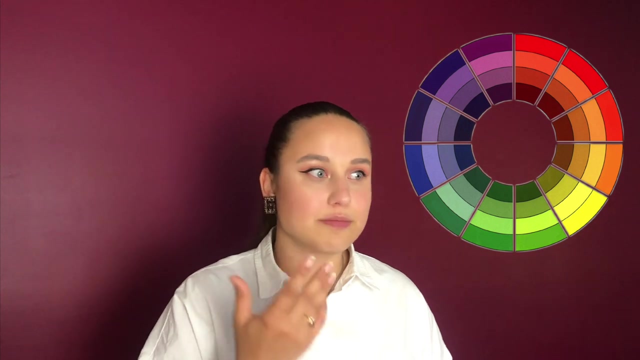 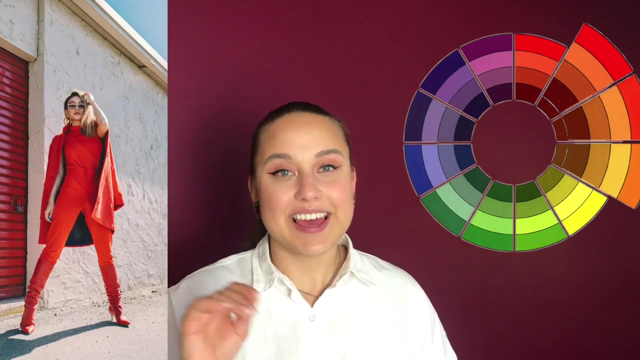 So the, the amount of the of the color can also vary. stay and like a one color category. So, for instance, if you choose red, just choosing the two colors that's closest to it would suffice. It's going to be a really nice. 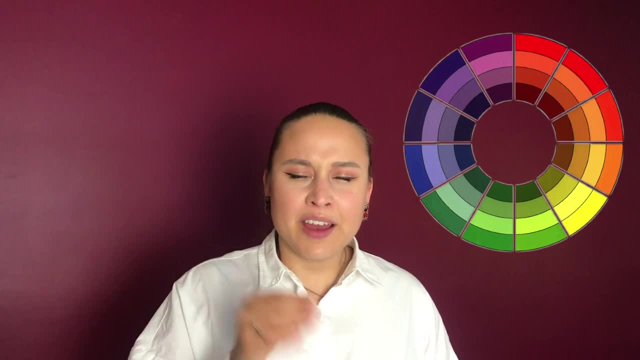 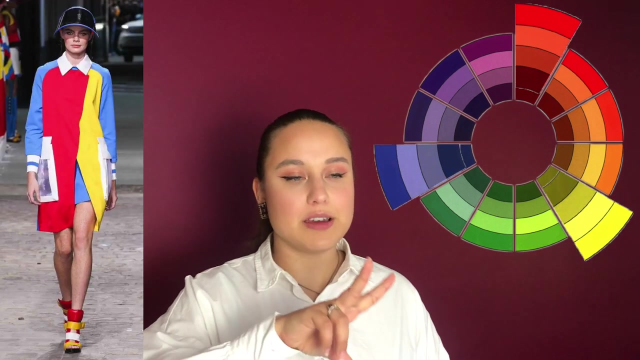 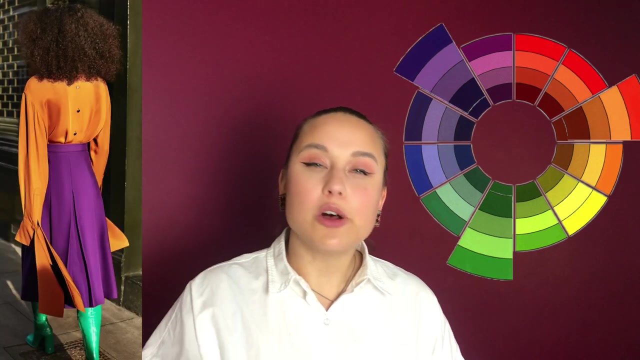 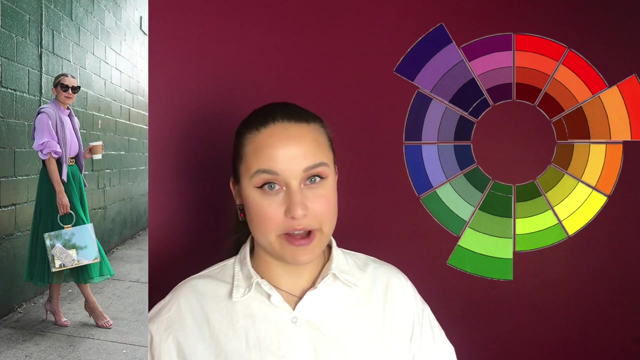 and simple vision. too complicated for the eye, excuse me. so the next kind of a thing, a color combination, it's called the triad, is the three like evenly spaced out colors on the color wheel. this is can also be a really bright combination and maybe you could choose to only you draw like wear the two and not 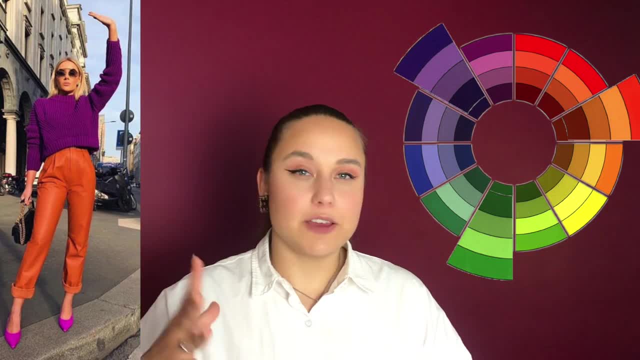 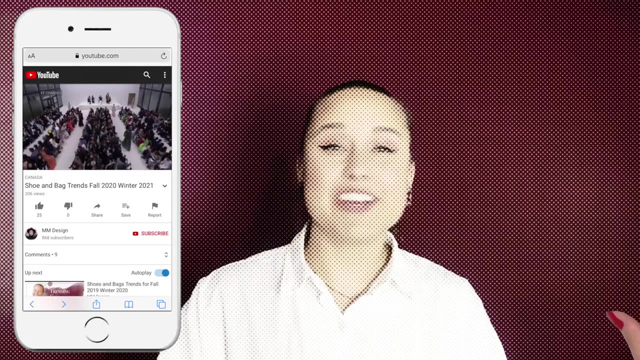 the third, just to tone it down a little bit. if you're thinking of wearing super bright, then go ahead. it's, you know, it's, it's none of my business. if you guys are enjoying this content so far, please consider subscribing and liking this video, thank you. 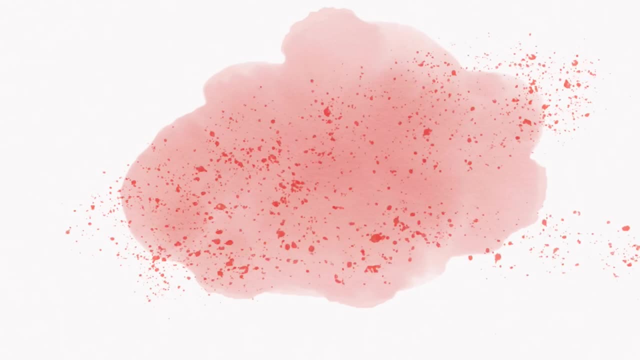 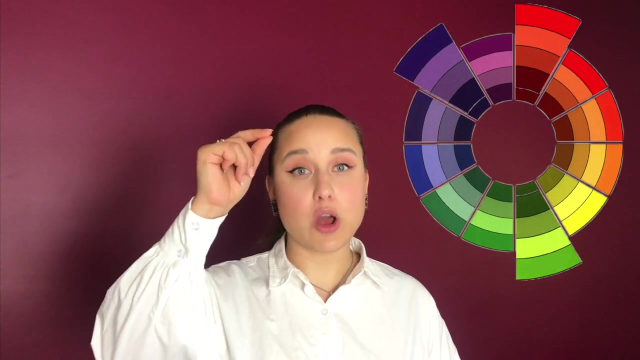 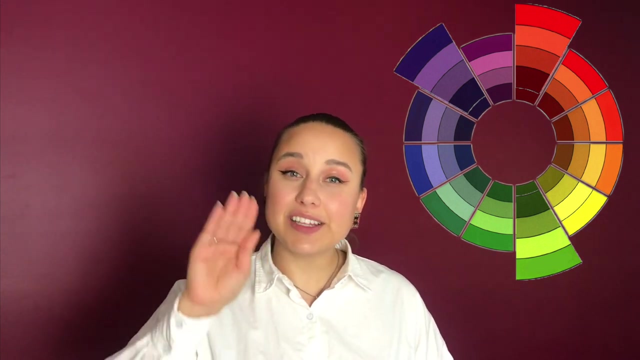 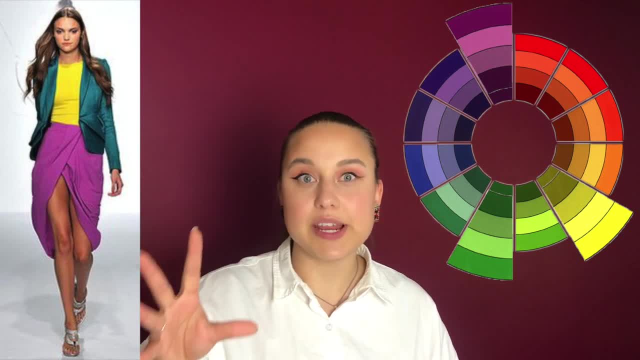 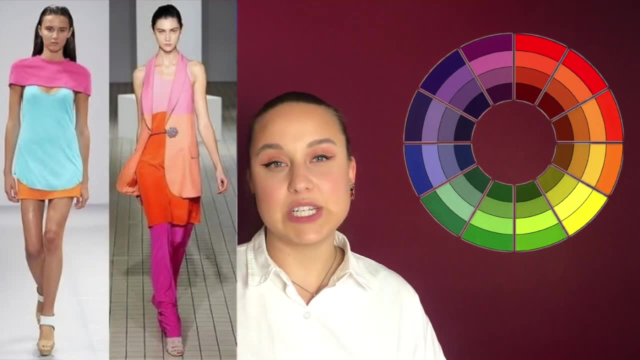 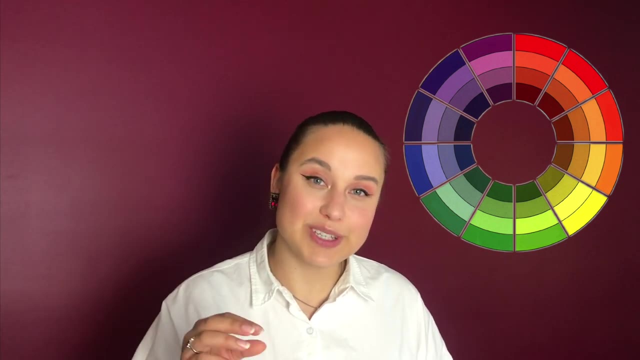 little bit lesser, of a like extreme combination of the complementary colors, but it is still quite bright. so if you're thinking of dialing it down, maybe try to use the tint or the shade of that of those colors together. so if you're thinking of dialing it down, maybe try to use the tint or the. 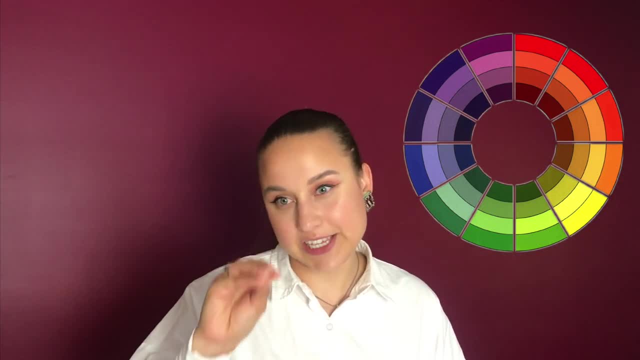 shade of that, of those colors together. so if you are not feeling like dressing up super bright, if you are not feeling like dressing up super bright, if you are not feeling like dressing up super bright and out there, then you can always tone and out there, then you can always tone. 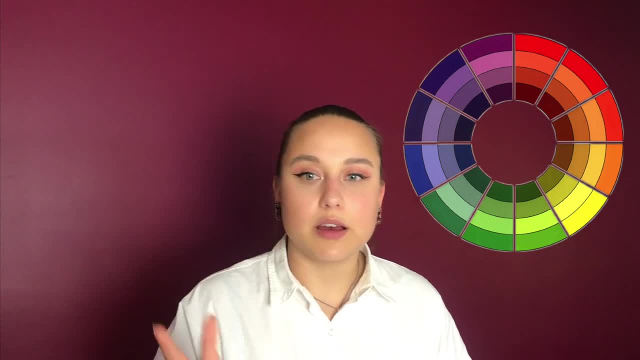 and out there. then you can always tone the colors down with neutrals like the. the colors down with neutrals like the. the colors down with neutrals like the. browns and nudes complementary colors. browns and nudes- complementary colors. browns and nudes- complementary colors. when they're mixed, they create a brown. 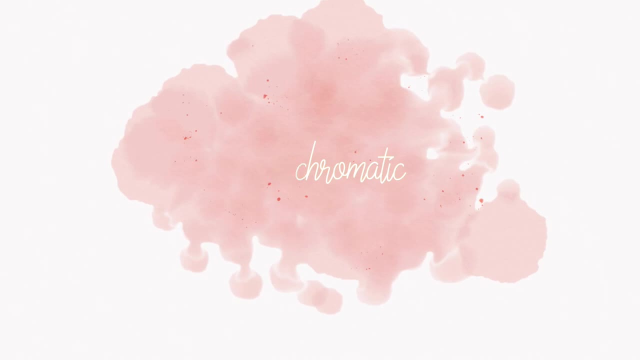 when they're mixed, they create a brown. when they're mixed, they create a brown color. there's different ways of dressing with. there's different ways of dressing with. there's different ways of dressing with color. you can go monochromatic, which is color. you can go monochromatic, which is 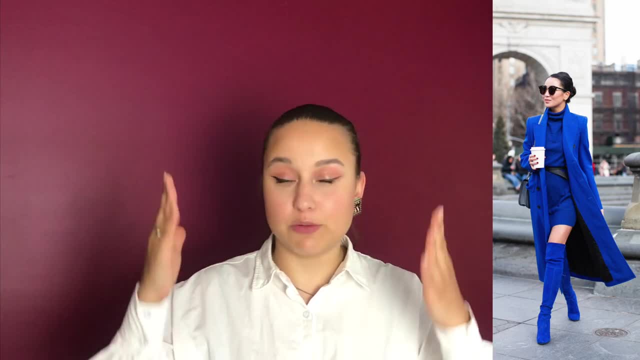 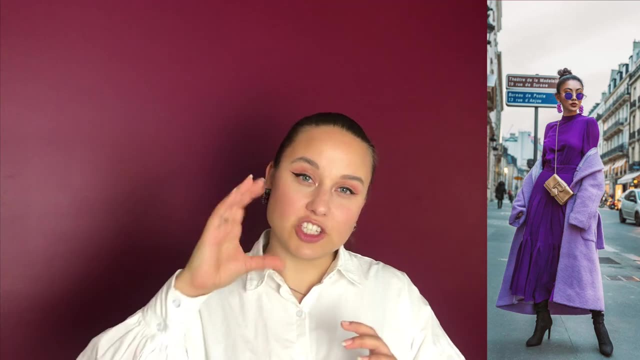 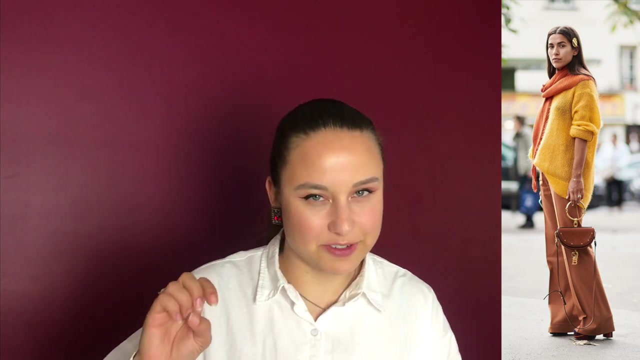 basically one color in different. it can be one color throughout, or it can be one color in different, kind of like a tint of that color, a shade of that color, a hue of that color. so it's one color but different strength of that color. if you know what i mean, i'll have some examples here so you'll. 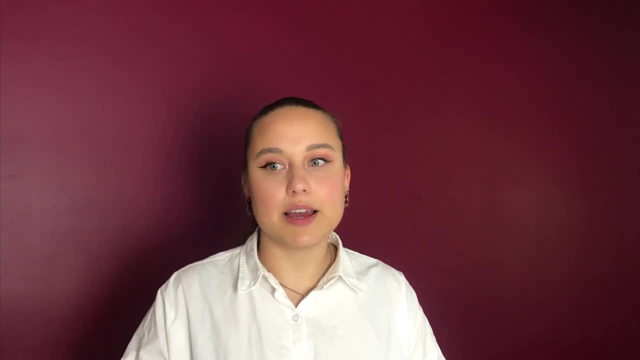 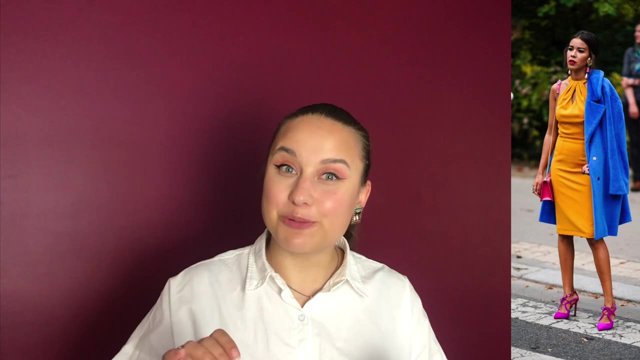 totally know what i mean. okay, so next one would be a kind of matching colors by the one, the thing that i was talking to you about by the circle. if you want to wear the complementary colors but you don't want to stand out as much, you can always dilute one of the colors or both of the colors. 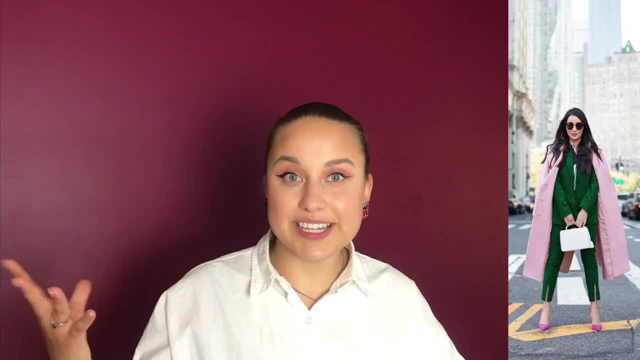 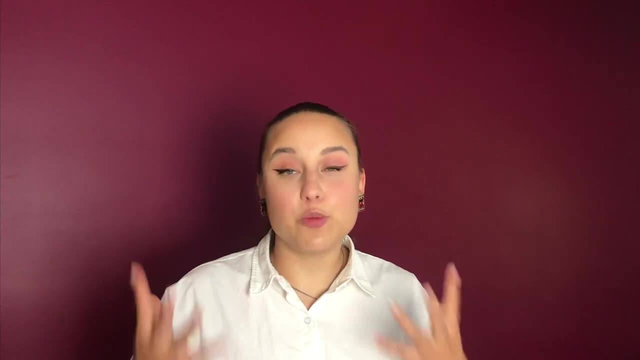 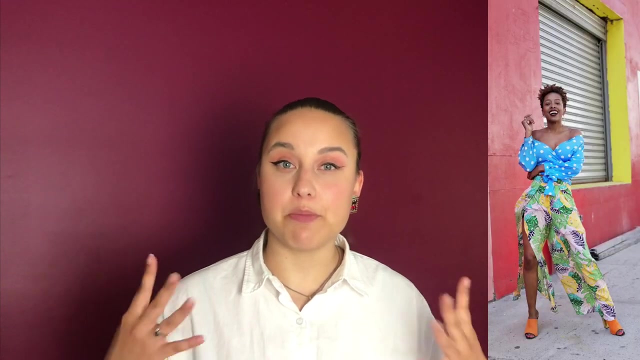 and make them either a shade or a tint of that hue that we're talking about. in the worst case scenario, you can always rely on prints on your garments. so, for instance, if you already have a print and it has different strength of that color, you can always dilute one of the colors and make them either a. 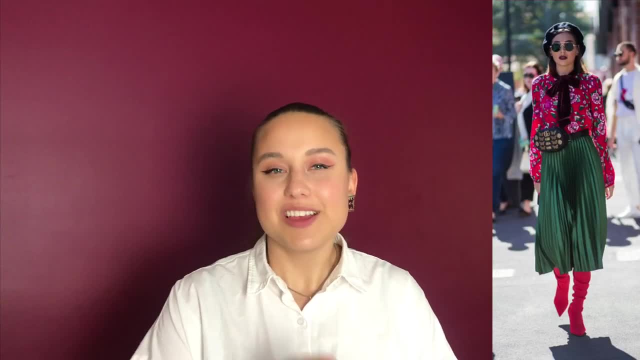 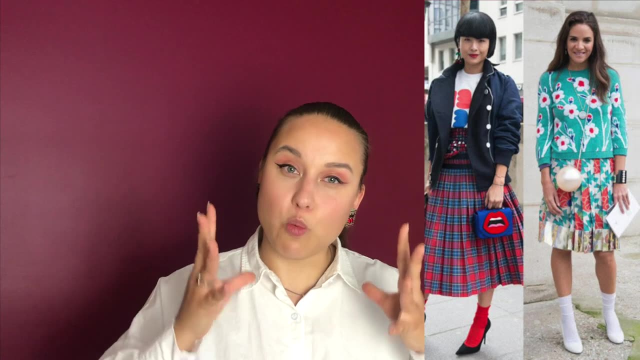 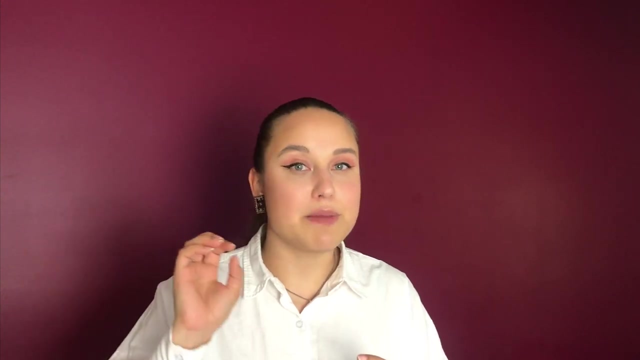 different colors, then you know for sure that these colors work together, so you can just pull one of those out and get more pieces of that color into your outfit. that way it's going to be like a one continuous cohesive outfit. you could also dilute that color and make it a lighter one, or make maybe 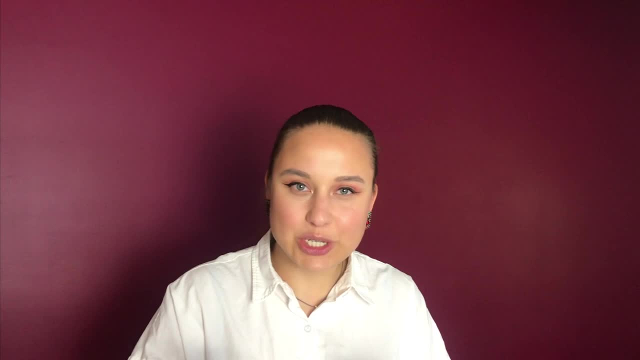 make it more neutral by adding, you know, gray to it, or maybe having it dark, like just darker. yeah, yeah, some of the prints may include those complementary colors, the ones that i'm just telling you kind of like, if that they may be too much, but they are used in different proportion. 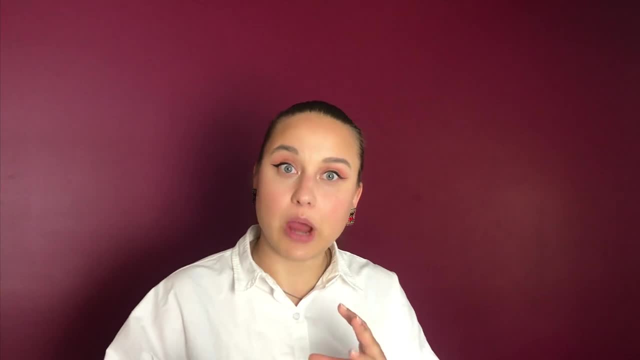 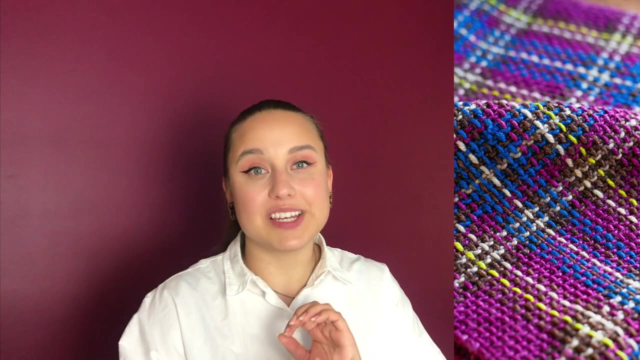 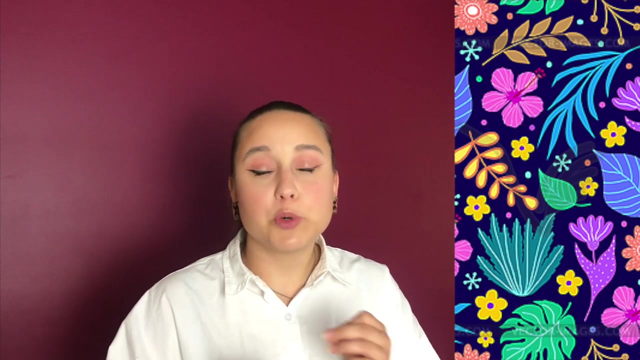 which is really important to see and figure out, because if they were used together in the same amount then it would be too much. but if it's just, for instance, a blue background and it has some- i don't know- purple purple flowers, and those purple flowers have little tints of that orange, yellow color that. 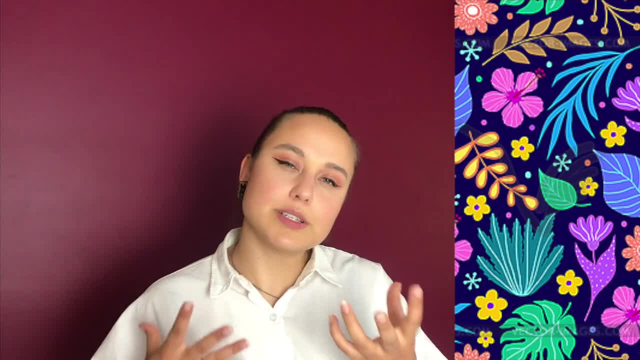 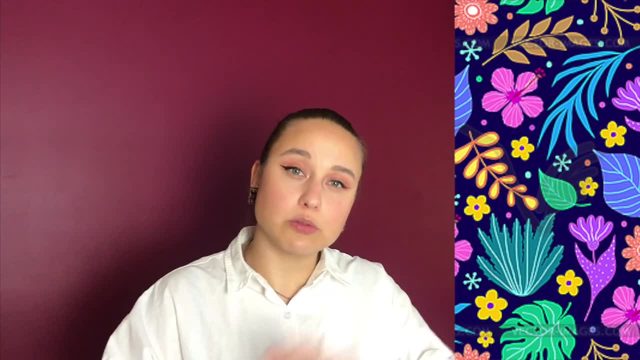 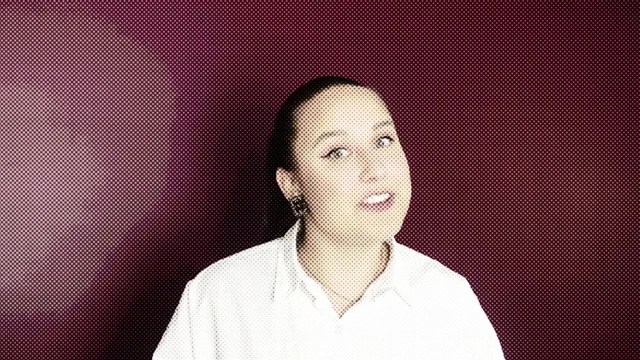 the complementary to blue. it's not gonna stick out as much as you know if it was those yellow orangey flowers on the blue background. if you guys are really scared about starting to wear print, or maybe you just want some more inspiration about how to do it, here is a video about how to start. 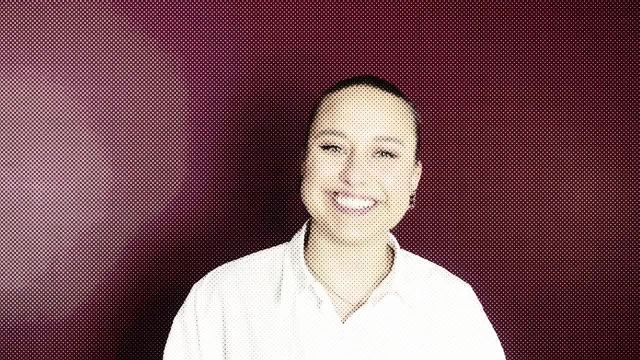 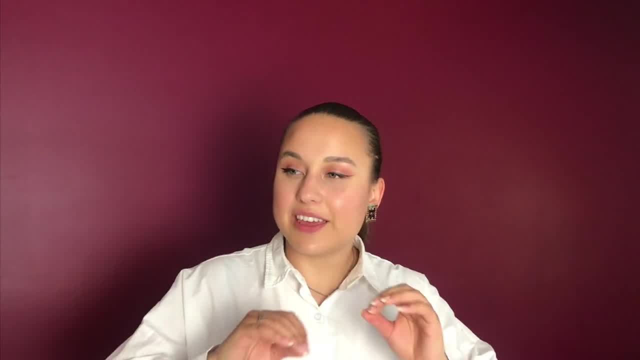 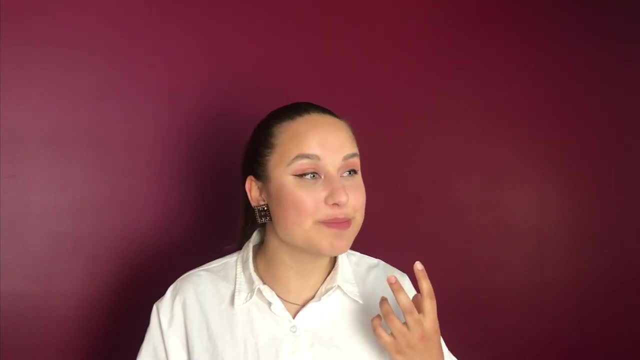 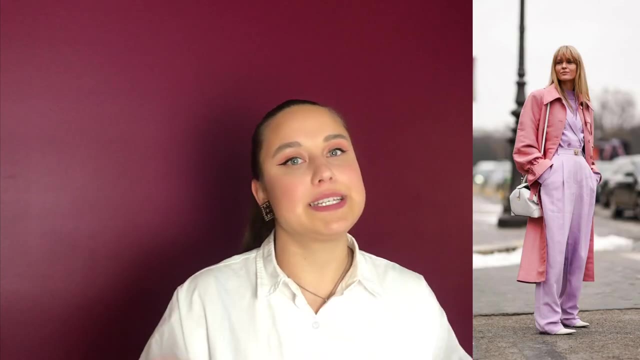 wearing print and how to just continue doing it. you okay another way of wearing colors. it depending on, like your style and how right you like the colors, or her sad, how subtle you want them to be. so wearing different colors in the same intensity. so, for instance, wearing pastels. all together, pastels are the tint of the hues that you're. 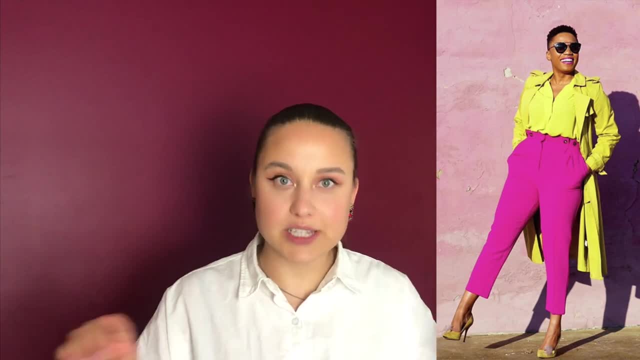 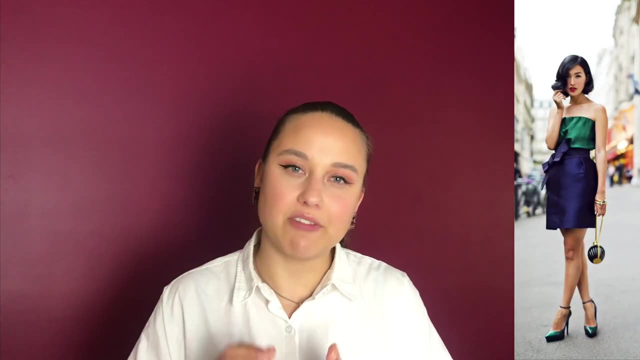 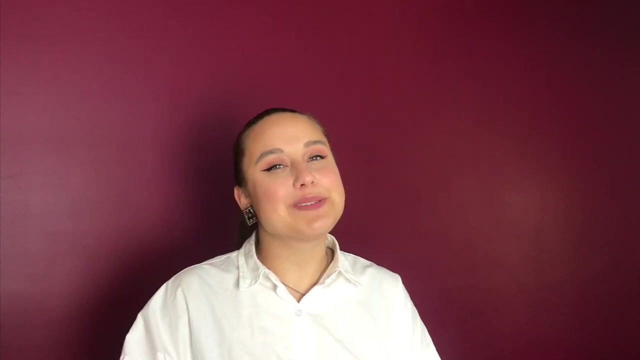 wearing or maybe wearing just really bright hues all together, or maybe wearing a jewel tone. so jewel tones are usually a little bit deeper. they have a little bit more black into in it, so it's more of a shade of the hue. all right, you guys, i hope this was useful. i hope you learned something new today and i hope you have a great day. stay classy. bye.